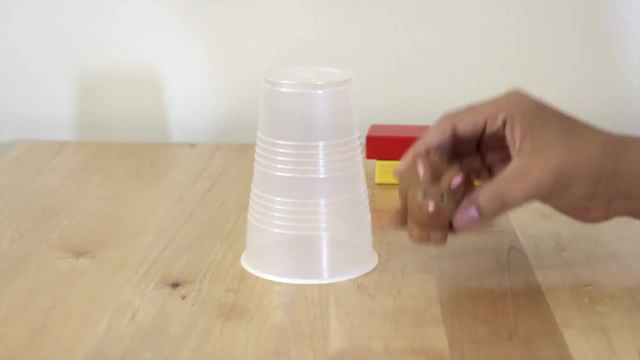 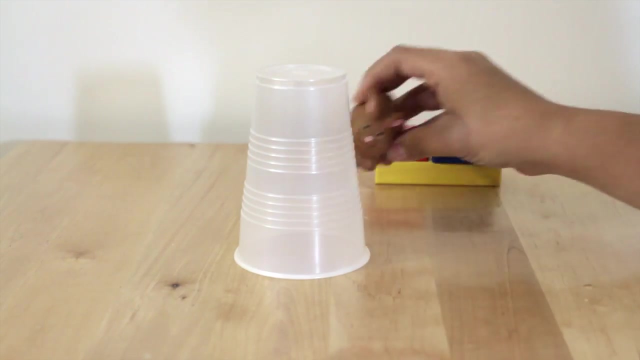 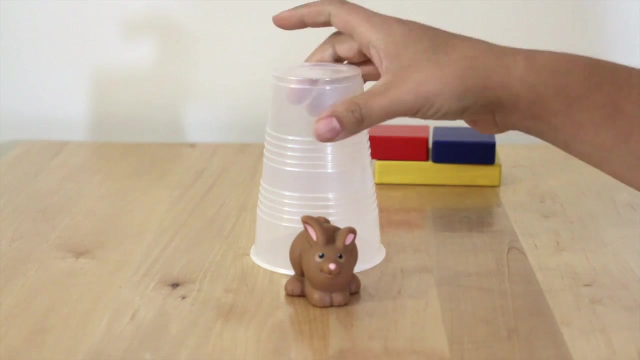 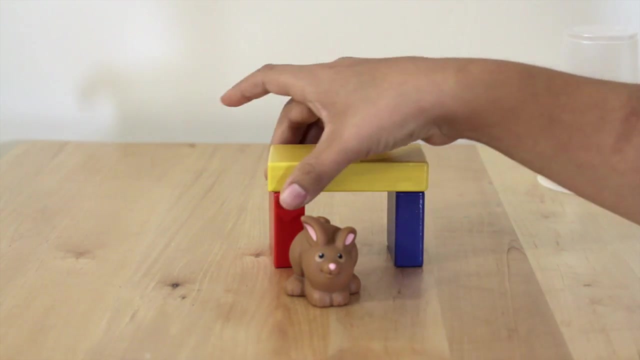 cup Same concepts: The bunny is on top. You can even do the bunny is inside or under. The bunny is behind And the bunny is in front. So just some things you can do to explore language and to teach these spatial concepts about what is above, beside, under, on top of beside. 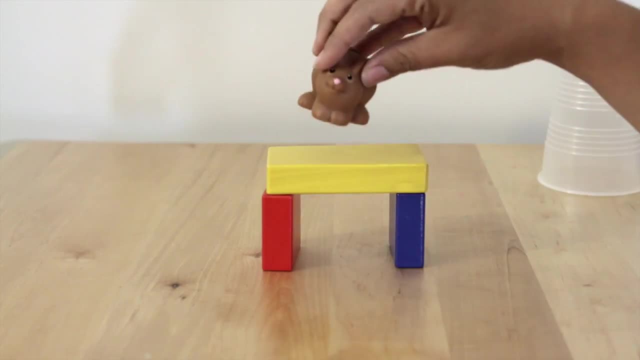 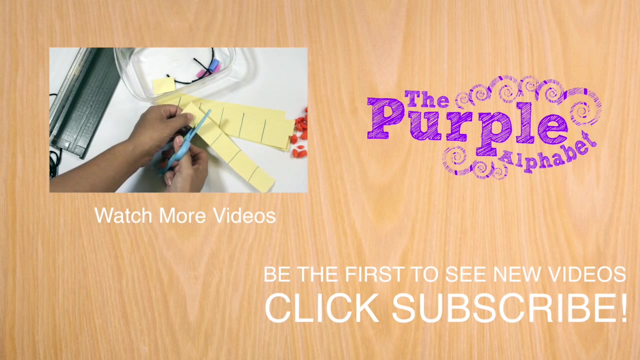 That's all for today, guys, Click subscribe to see some more videos like this. Give me a thumbs up to show your love And I'll see you next time. Bye-bye. 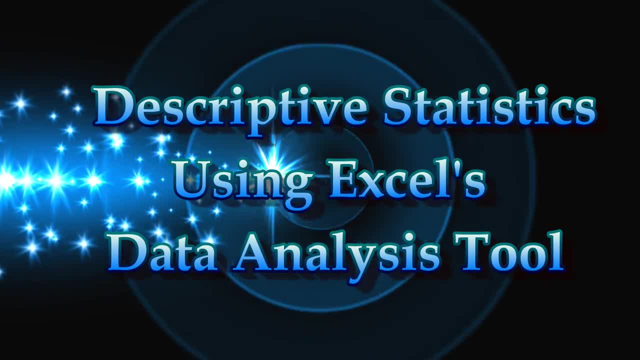 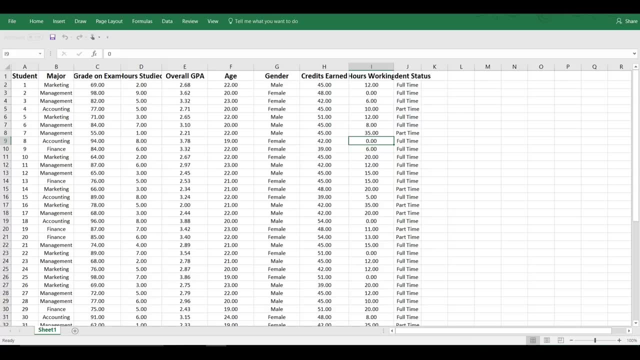 Welcome to this tutorial on how to calculate descriptive statistics using the data analysis add-in tool. The first thing you need to do is to make sure you have the data analysis tool installed on your ribbon, So let's click on the data tab and see if the data analysis 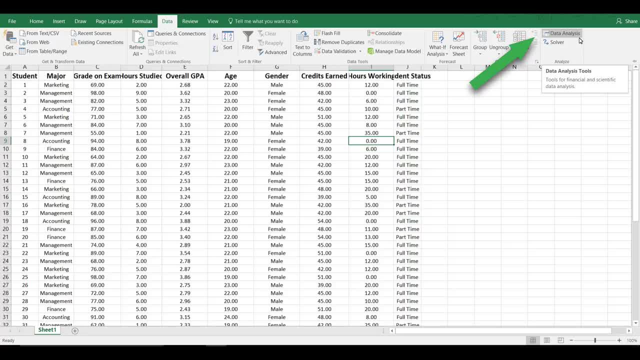 tool is there and it is right here. As you can see, I have already installed this. since I've done this before, You only have to install the data analysis tool one time. By default, Excel comes without it installed to save memory, So once you install it, it will stay there. 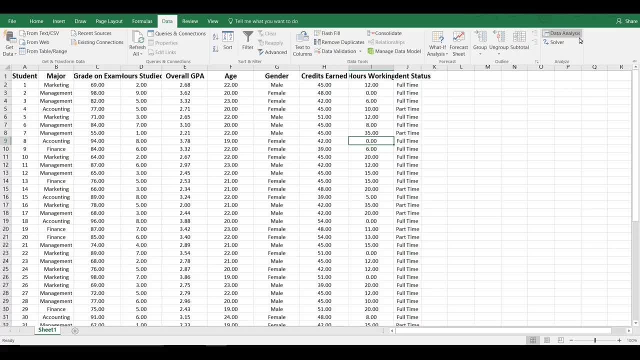 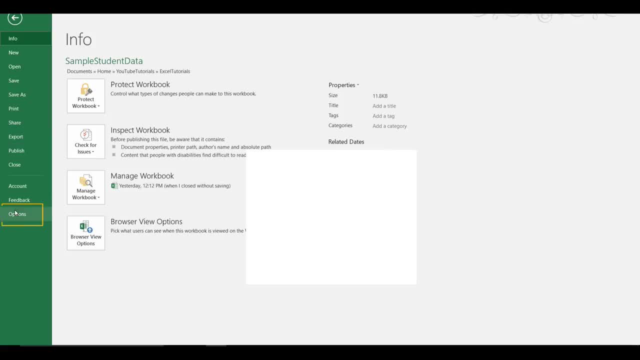 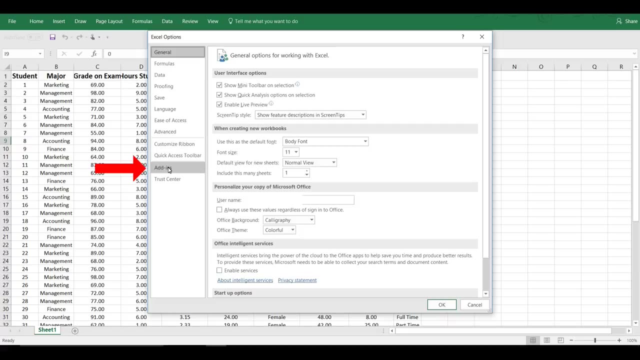 If you see that the data analysis tool is not there, then you need to add it in. To do this, go to file, scroll down to options, click on add-in and then click on save, So you will see the options in the Excel options dialog box Once you've clicked on the add-ins. 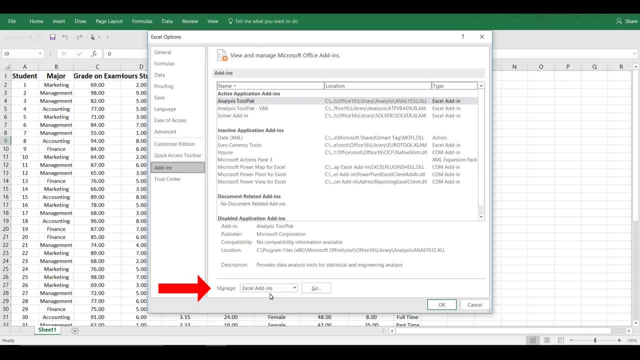 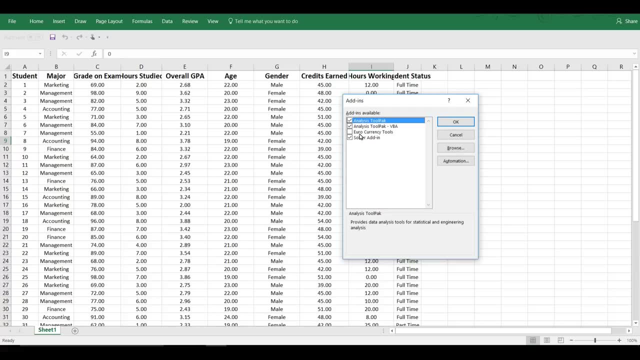 you will have more choices. Look at the bottom where it says manage Excel add-ins and click go Now in the add-ins tool box. you see there are check boxes. I already have analysis tool pack checked. If it's not checked, make sure you check it off and then click okay And